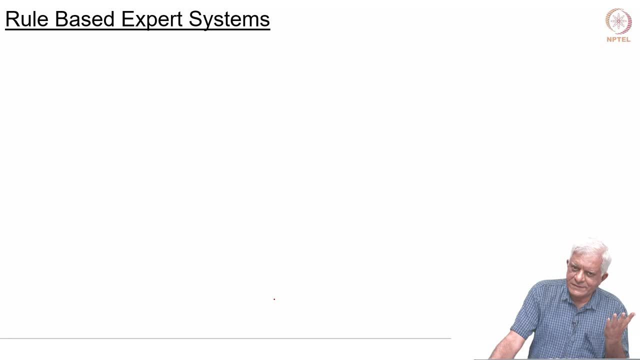 And they wanted to implement applications in various domains. and where do you get that knowledge from? that something implies something else. They said we will go to the experts in the domain and they evolved the whole approach of knowledge acquisition that they 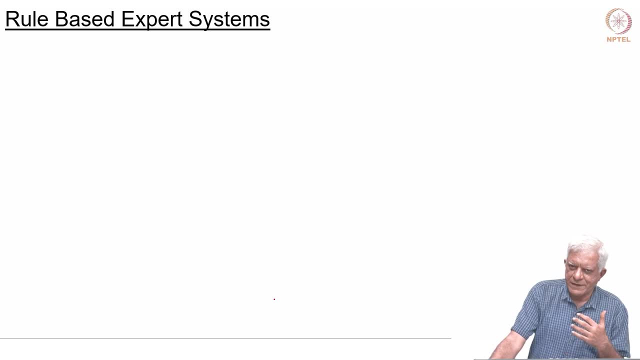 would interview them and somehow extract the rules from them, and they would extract the rules. That is why they are called rule-based systems. They call them expert systems because the rules were extracted from experts and the hope was that the program that they build would perform like a human expert. essentially, 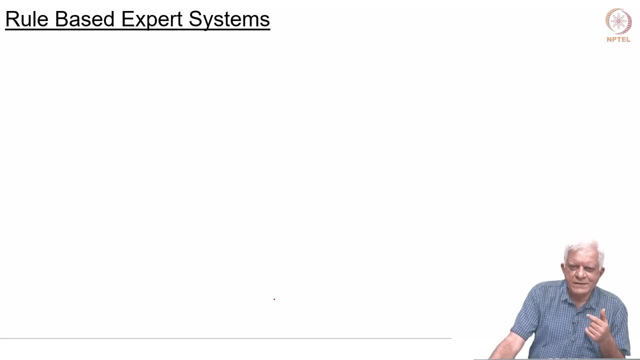 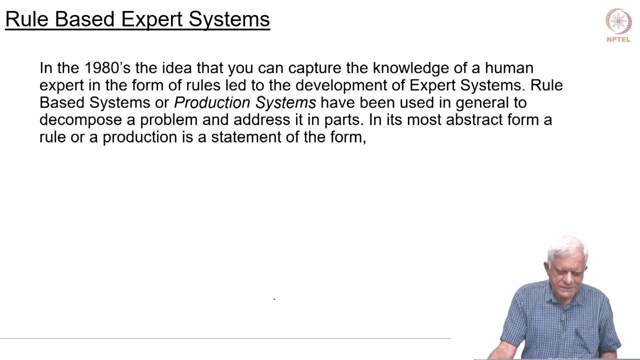 In some cases this was successful. in some cases it was not possible because it was difficult to extract the rules that people were using implicitly, but nevertheless it was a very successful process, successful phase of application of this, this thing, And it used this notion of rules that 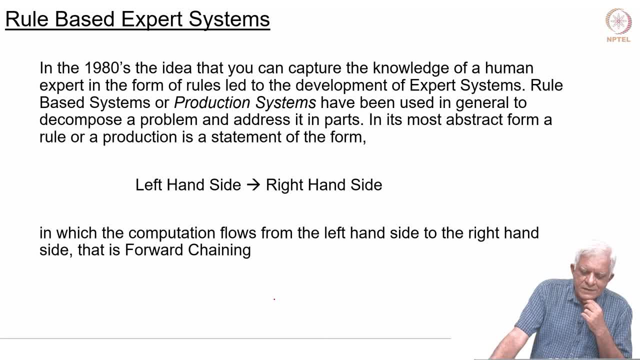 is why we are bringing it in here essentially. So, as I said in the eighties, the idea that you can capture the knowledge of human experts in the form of rules. this rules is important essentially, and you know that is where we are making inferences led to the development. 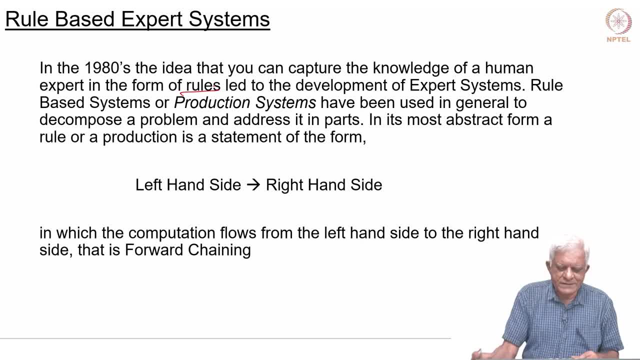 of expert systems, Rule based systems, or production systems as they were called, were used in general, in general to decompose the problem and address it in parts. essentially, Every rule would express, would kind of address a part of a problem and eventually, if you had a whole, 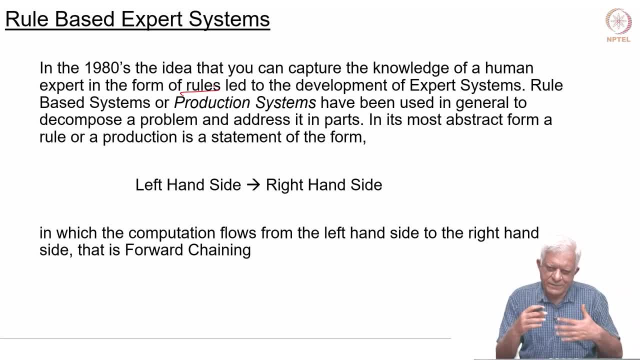 bunch of rules and you had a problem. then you know, eventually, by applying rules, different rules, it would get solved. that was the idea. The rules would come from experts, essentially. So, in the most abstract form, a rule or a production is a statement of the form left. 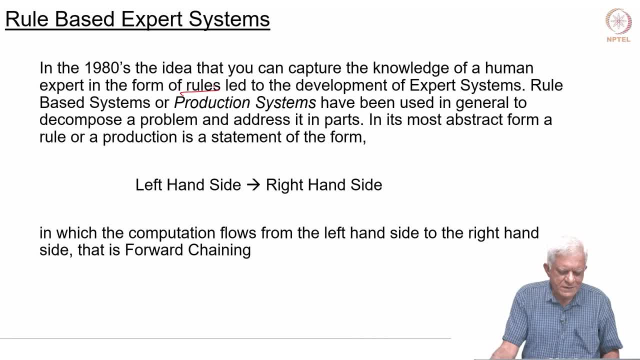 hand side, right hand side, which is like an implication statement, in which the computation flows from the left hand side to the right hand side, which is what we are calling as forward chaining. So if you know the left hand side, then you can kind of conclude the. 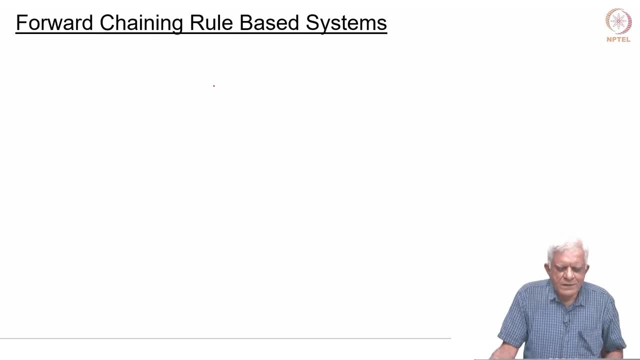 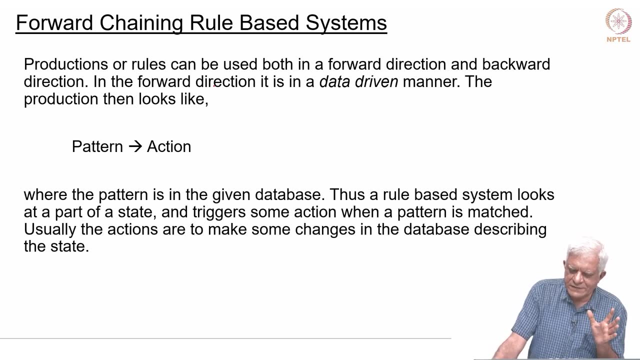 right hand side. In practice, production rules can be used both in forward direction and backward direction. So what we are going to do is we are going to use the rules of the left hand side. So once we are done with this rule-based introduction, we will actually move towards backward reasoning. 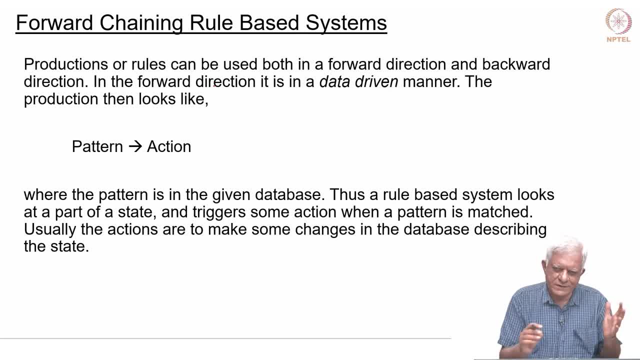 or backward chaining, and we will see that that is another way of doing inferences which has its own advantages, And in fact, rule-based systems were also built in backward chaining, and we will look at a language called Prologue which does backward chaining essentially. But 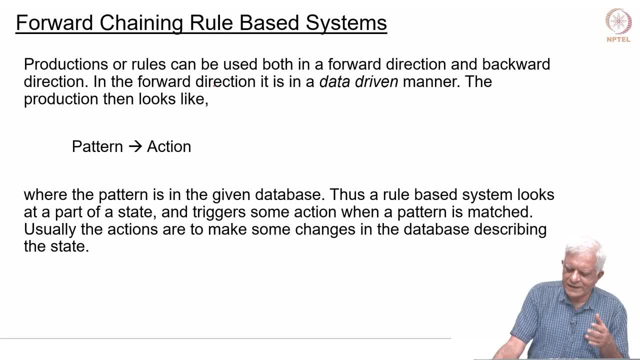 in general. we are now looking at the data driven aspects. So in the forward chaining aspect of it, which is forward chaining, the production looks like pattern followed by action. in the forward chaining context, In the backward reasoning context it is more logical: The pattern is in the given database and the action 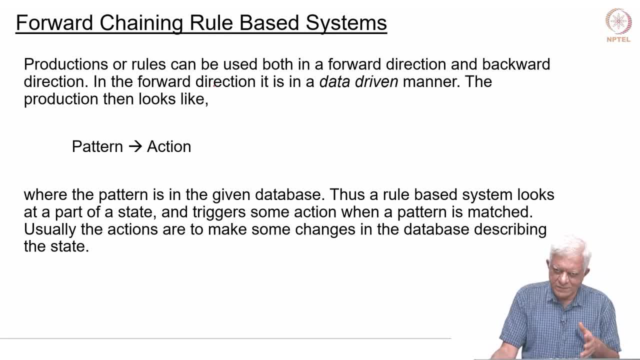 could be something: add a new statement or even delete a new statement. We have not talked about deleting statements here, but in rule-based expert system you could delete statements And that ends up in a, you know, slightly more complex logic, which is sometimes called. 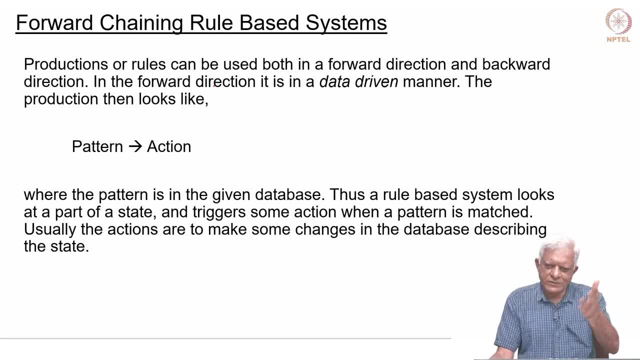 as a non-monotonic logic, Because you know you prove something and then you delete it later. then it is no longer true And that is why it is called non-monotonic. The set of true statements can go up and go down, and go up and go down, But we are not getting. 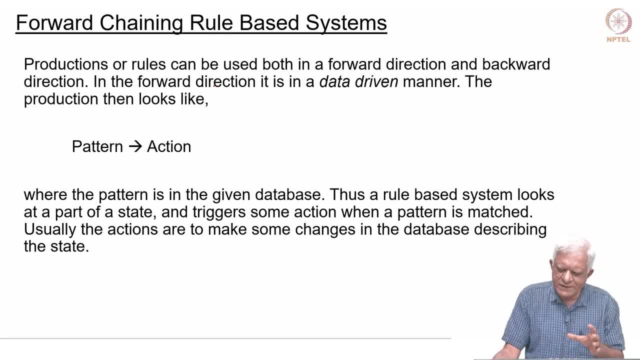 into that right now. We want to just look at this and connect with the fact that forward reasoning, forward chaining in logic is tied up to this expert systems area. So there is a rule: a system looks at part of a state, triggers some action. Then, when a pattern- 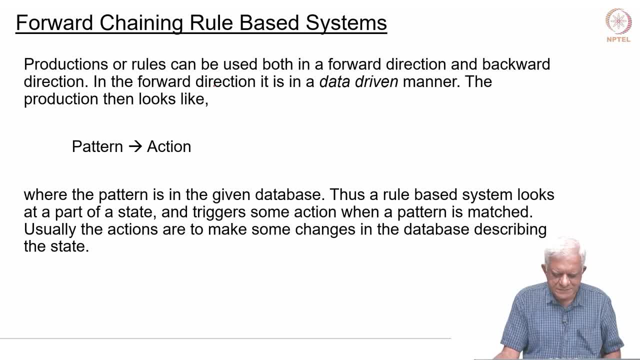 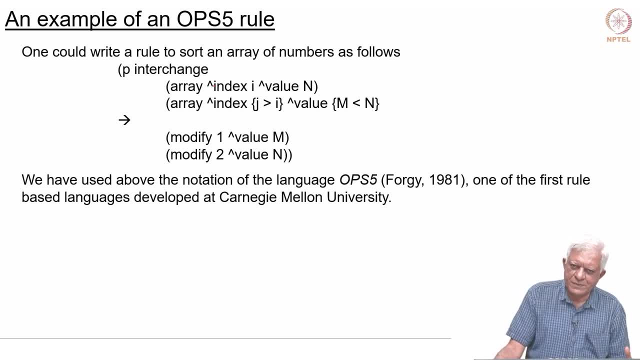 is matched and this process goes on essentially. Here is an example of a rule in the language called ops 5.. The ops 5 is, you know, somewhat ambitiously named as Official Production System Language. It was. it came out of CMU, where some of this work was done, as mentioned here. That depends very much on some production originally, or what is the benefit, or a risk, or the потому, the normal risk, Whether something is successful or not as well, which situation is emerging until a productive? 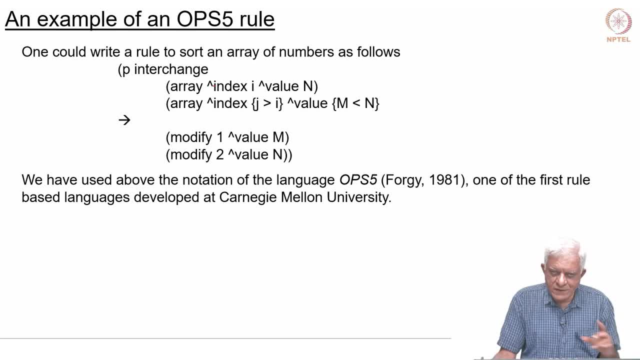 order is formed That will total essentially this rule, based on that rule and then it listening, And Charles Forgy, whose work we will see later in the course, was one who did this. But here we are not talking about expert systems or not, we are just looking at the language. 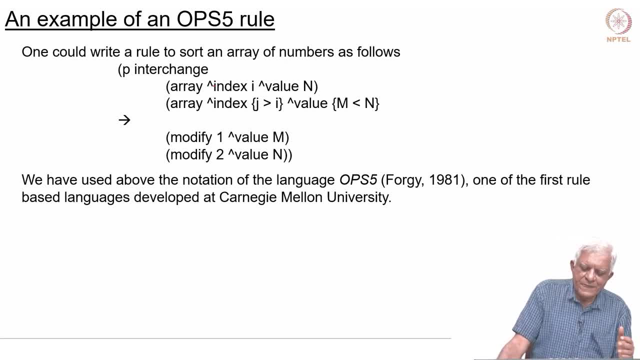 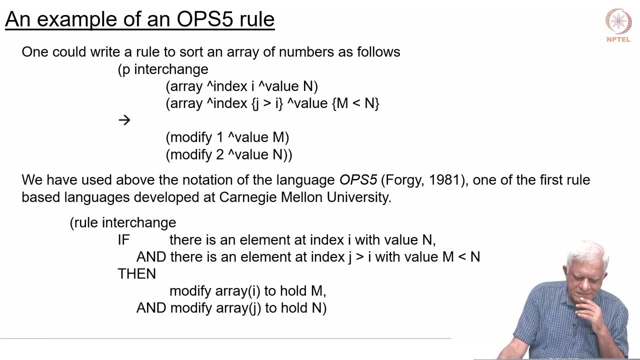 essentially, or the nature of a rule. So let us look at both the rule in English and in this ops-5 language. Let us call the rule, as it has a name, called interchange, And our task is to sort and edit, essentially So what this rule says that if there is an element at index i and whose value is n and 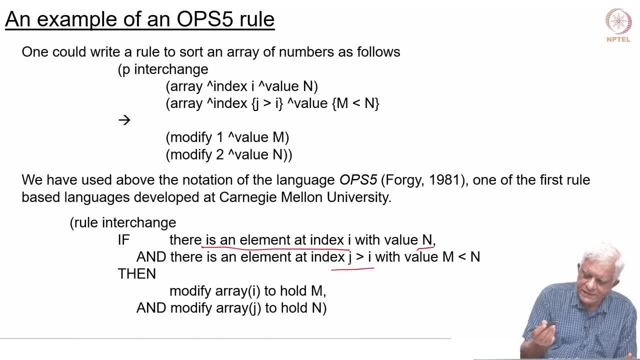 if there is another element at index j which is greater than i, but whose value m is less than n, then you just swap those two elements. Bring m to right. Okay, So bring m to index i and bring n to index g, so that the smaller number comes first. 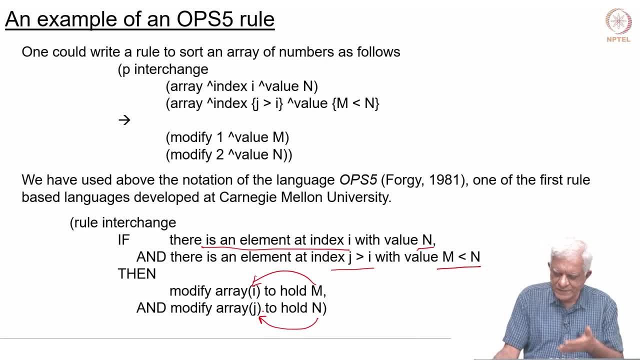 and it is an ascending array of numbers, essentially. So what this rule is simply saying: spot two numbers out of place and swap them. essentially as simple as that, And you can imagine, if you think about this, this one rule will actually sort your whole. 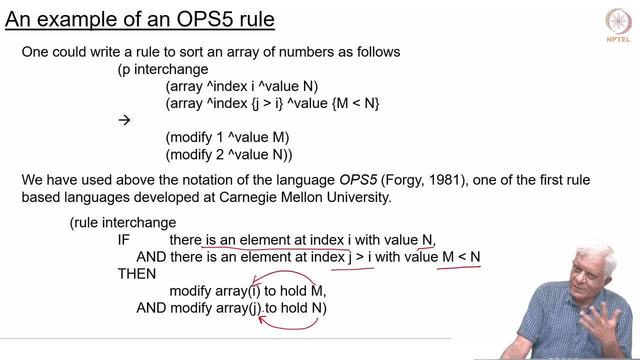 array. Just run it enough number of times, it will spot two numbers out of place and change them. Of course it will not be efficient and that is why we do not use this approach, but it will do the task for you. In this language of Swy, which is just a very quick introduction, we have this notation: 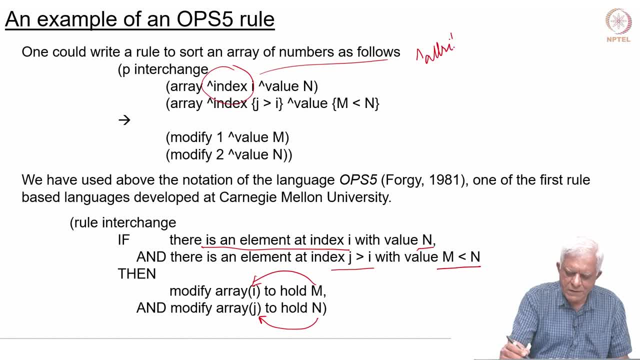 which is attribute And value. when I say value, I am even allowing things like relational symbols and things like that. essentially. So the same thing is said in this particular language: If in the array at index i there is a value n and if at in the array at index j, which 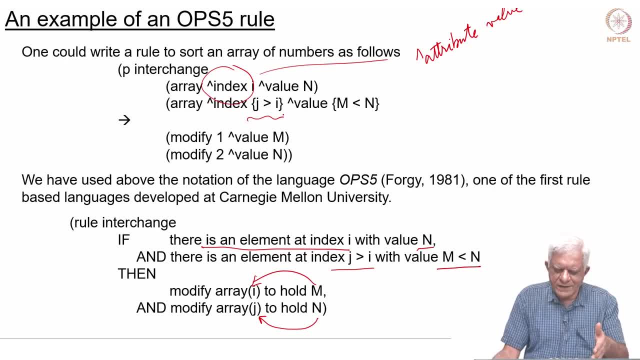 is greater than i, there is a value m which is less than n, Then modify the two values. If there are two locations, the first one should contain m and the second one should contain n. This is just an example of a rule, and there are many, many things you can do simply by 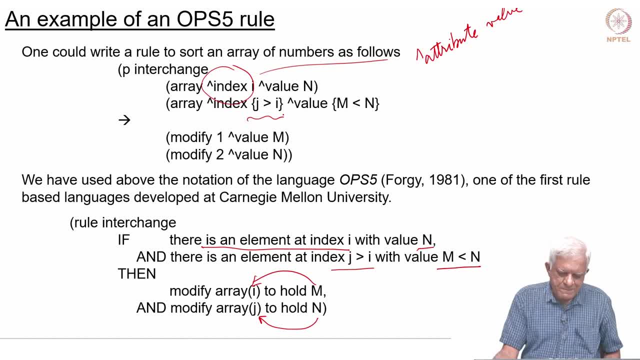 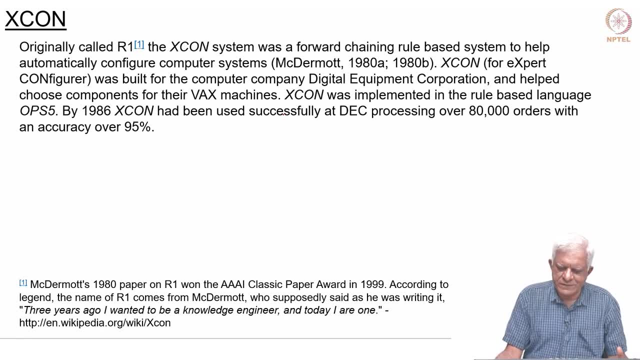 expressing your program as a rule, essentially. So. here is one system which was became very popular. This was called R1 or Xcon, Xcon meaning Xcon- It was a con- is for configuration and x comes from wax machines, which was a very 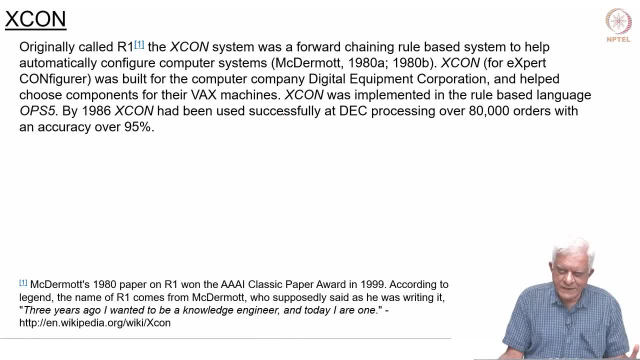 popular machine in the mid 80s: DEC wax. DEC was a company, Digital Equipment Corporation. What this program would do is that it would help people configure their machines that they were buying. In those days, machines were not As simple as going and buying a small mobile, which is a, which is a computer nowadays. 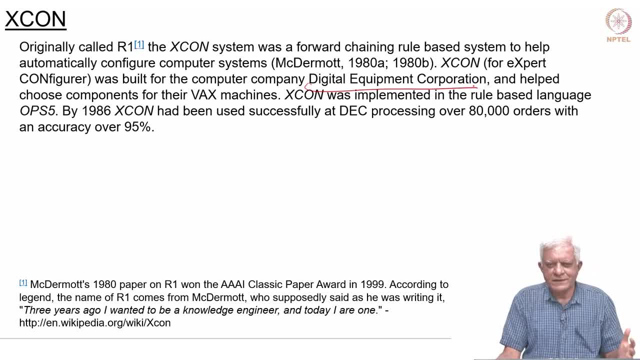 you had to, you know, have a room for the machine first and then put in your specs and get this whole big machine which occupied a significant part of a room. So he, this was written by McDermott. McDermott is the same McDermott who was part of you. 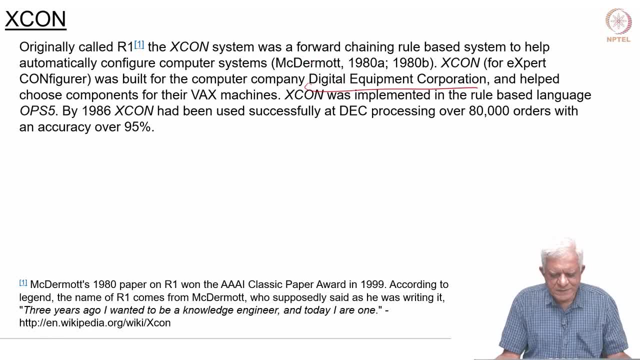 know Charniak and McDermott. He wrote a book which was very popular. He developed a forward chaining, rule-based system for configuring the computer systems. this thing- So okay, so I said wax- X stands for expert and con stands for configurator- was built. 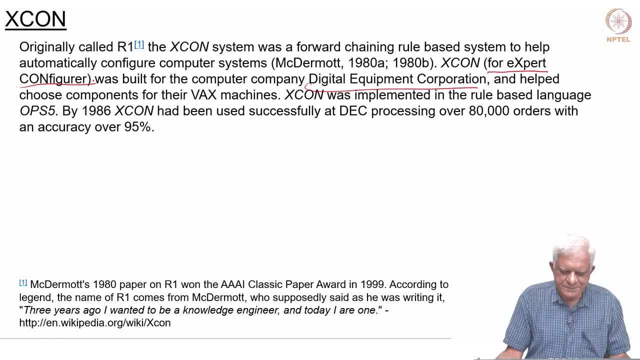 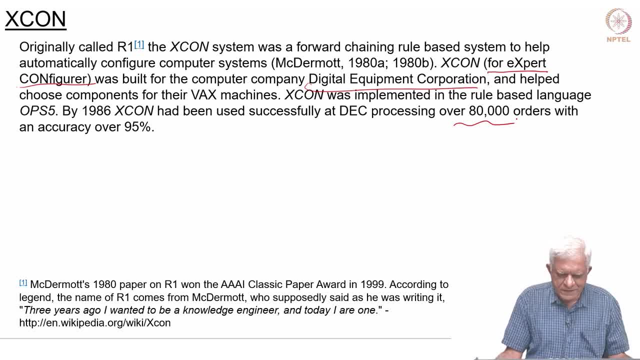 There is a small anecdote of why it was called R1 and then changed to Xcon. So some it is not clear whether this is true or not, but anyway, apparently McDermott, he said that three years ago I wanted to be an orders engineer and today I R1, so 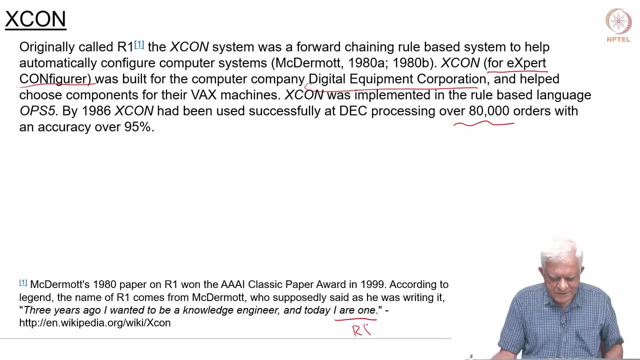 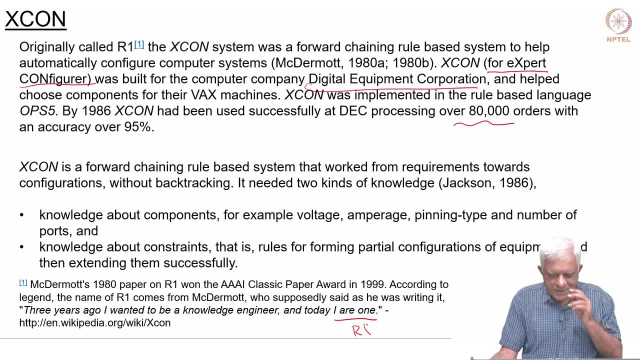 this R1 is where R1 comes from, but you must always take this with a pinch of salt. So it is a forward chaining, rule-based system that works from requirements towards configurations without backtracking. There is a nice book on expert systems by Peter Jackson, also written in 1986, and you 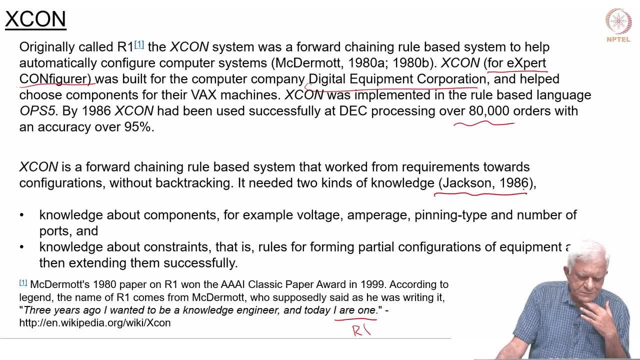 can read more about this if you get access to this book. So it had knowledge about components, for example. you know what are the specifications of every component, and knowledge about constraints, so you know how should components feed into each other. 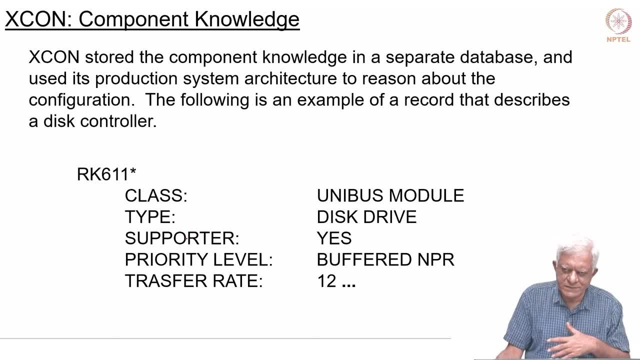 And essentially it did this whole process by this rule-based search. it is a kind of a search which it was doing, So it stored component knowledge in a separate database, and this is an example of the kind of knowledge that we are not particularly interested in. that it is just to illustrate. 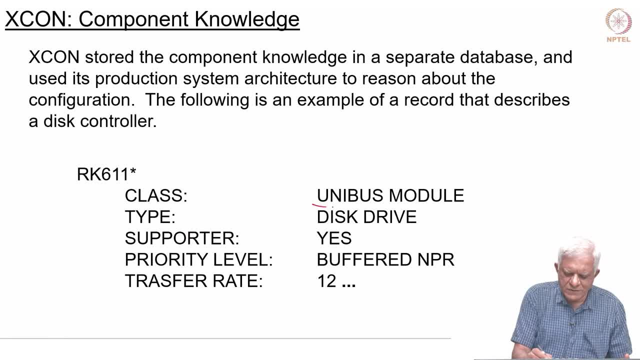 this idea that when you are talking about a universe module, then it is of a type disk drive and it supports something buffered- NPR, whatever, whatever. So it is a kind of a search. So it is a kind of a search which it was doing. 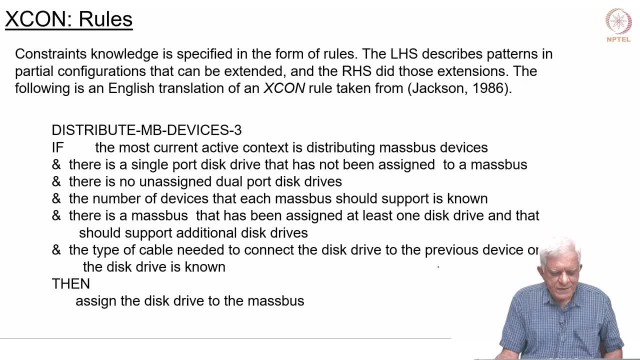 And rules were of the if-then kind. that is what we want to illustrate here, this thing. So this rule says, for example, if the most current active context, this context was an idea used in OpsWave to channelize computation, because if you have hundreds of rules, which 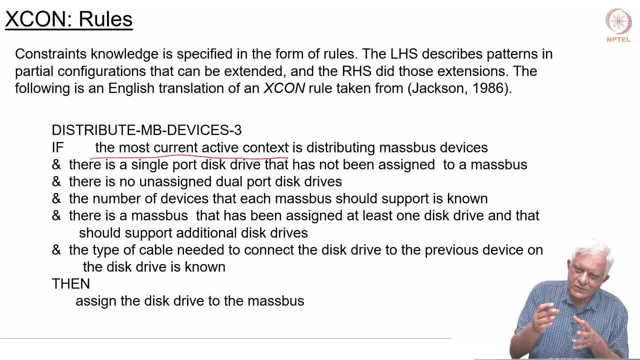 rules do you match? So the language allowed. So you have to set context and say: in this context, only these rules are applicable. So if the context is distributing mass-based devices, then if all these conditions are true, which we will- I will not read out, you can read them at leisure- then assign. 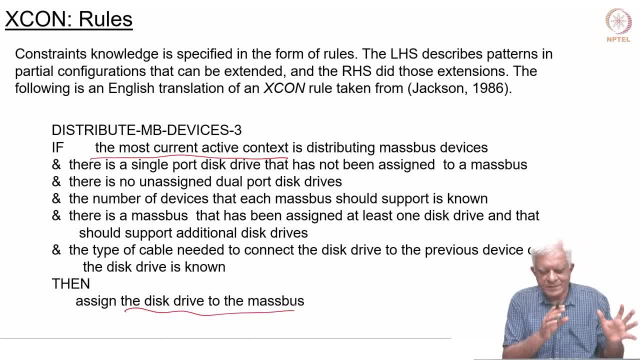 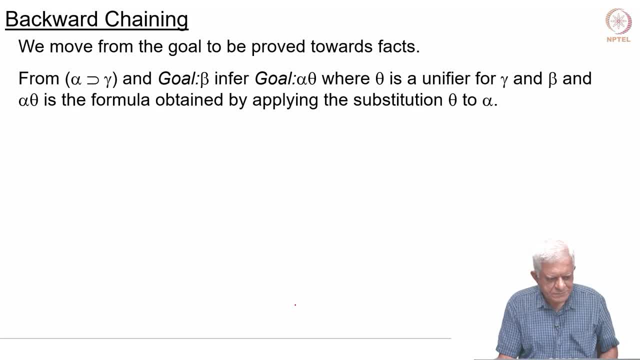 the disk drive to the mass processes. So if these conditions are met, then you will say that ok, this is a disk drive that we are using, and so on. So that was a very quick introduction to OpsWave. Thank you. 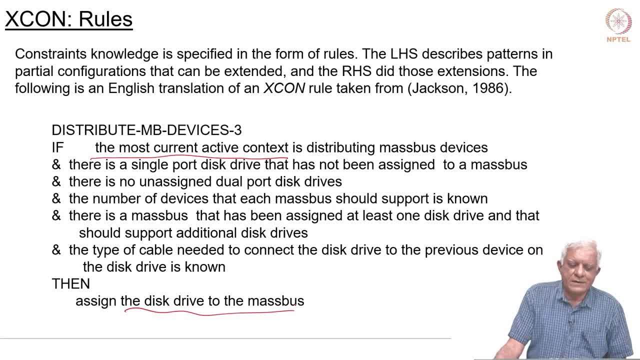 Bye. So rule-based systems. we will come back to rule-based systems. in fact, we will come back to forward chaining, rule-based systems and we will look at this work of Charles Forgy, which said that if you have these hundreds of rules and if you have these hundreds of